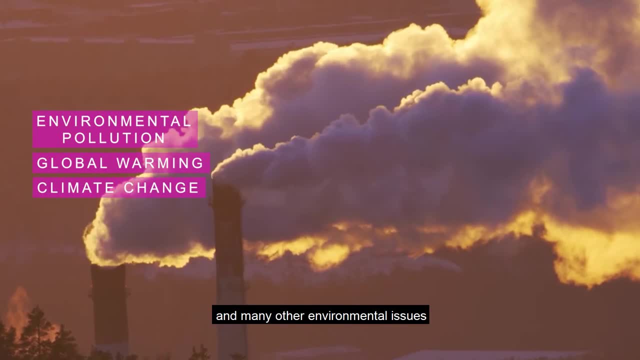 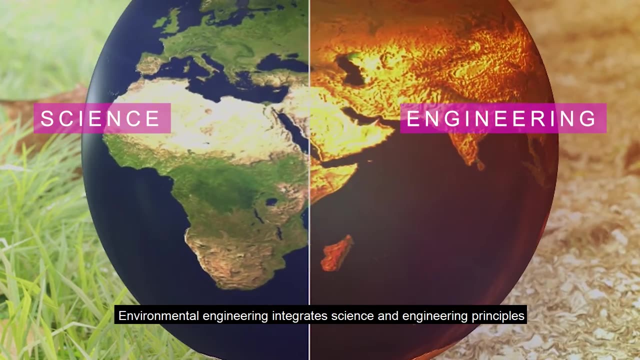 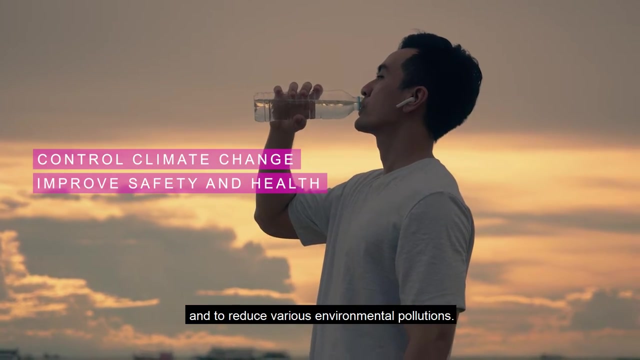 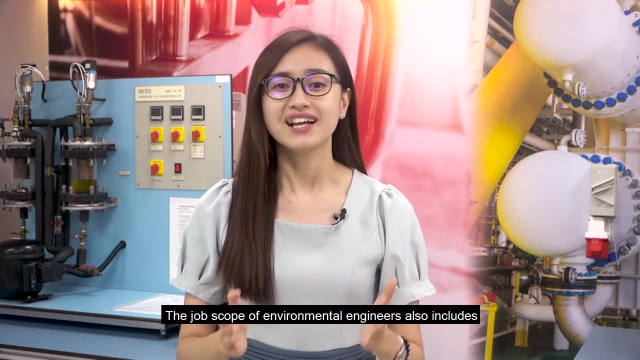 global warming, climate change and many other environmental issues that we currently face. Environmental engineering integrates science and engineering principles to help us to control the climate change, to improve the safety and health of the people and to reduce various environmental pollutions. The job scope of the environmental engineers also include designing. 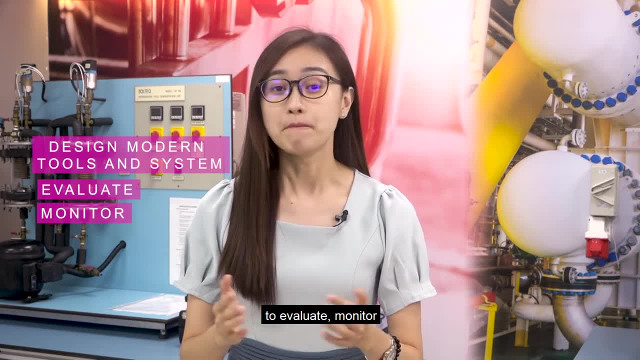 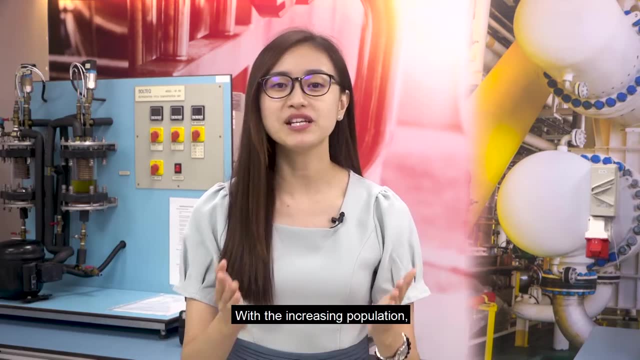 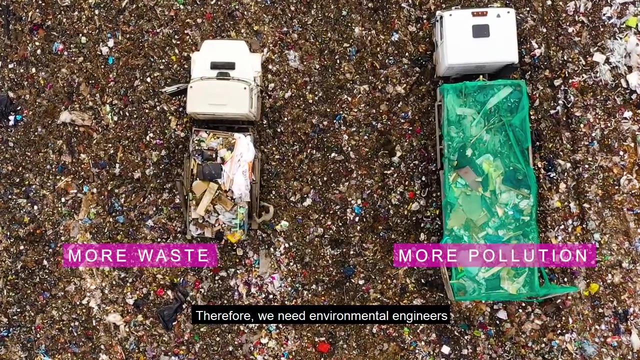 of the modern tools and systems to evaluate, monitor and reduce environmental risks and the impact from different engineering projects. With the increasing population, they will be more waste and there will be more pollution. Therefore, we need environmental engineers to help us to deal with the rise of the pollution and to maintain a safe and healthy environment. 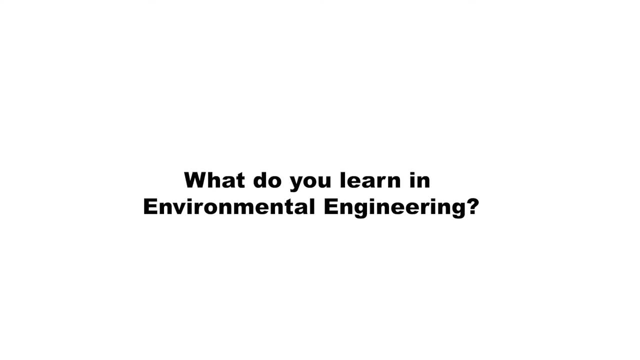 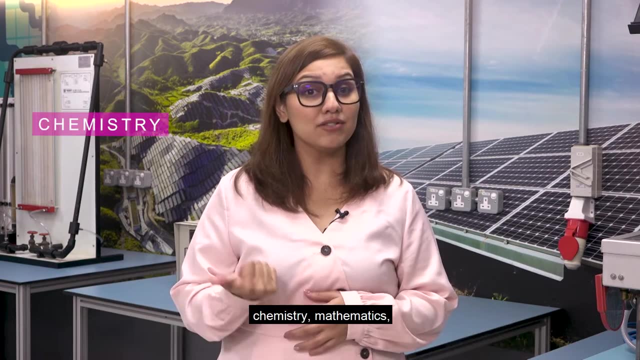 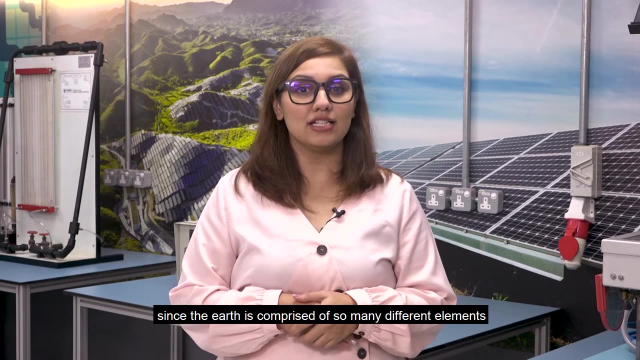 and society Generally. environmental engineering is a combination of different fields which involves chemistry, mathematics, biology, ecology, geology, hydrology and many more. since the earth is complex, Environmental engineering is comprised of so many different elements, such as air, water. 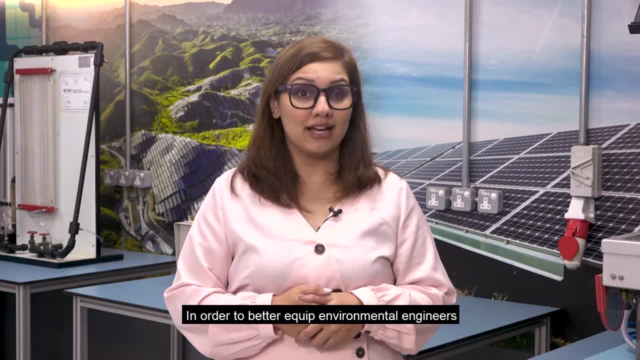 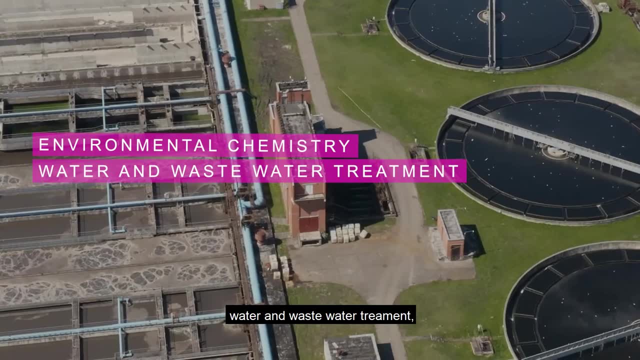 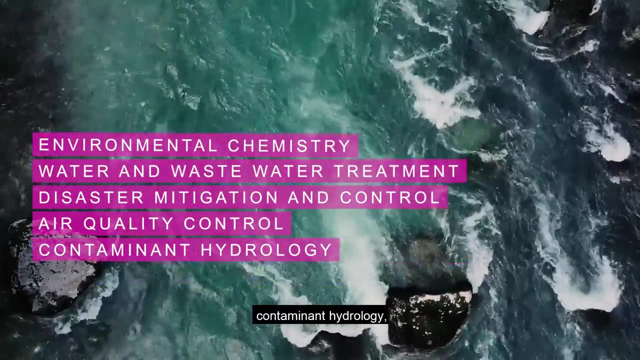 and soil. In order to better equip environmental engineers to treat pollution, the students in this programme would undergo courses such as environmental chemistry, water and wastewater treatment, disaster mitigation and control, air quality control, contaminant hydrology, water efficiency and conservation, and many more. Environmental engineering also focuses 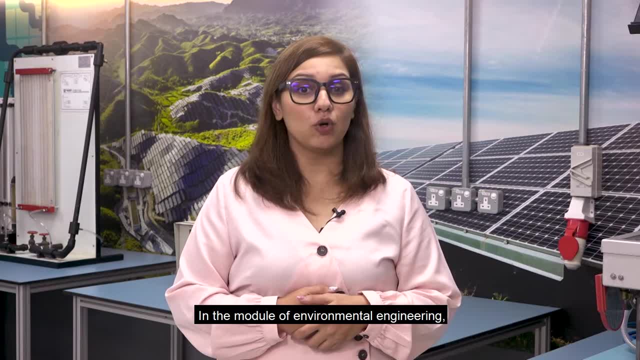 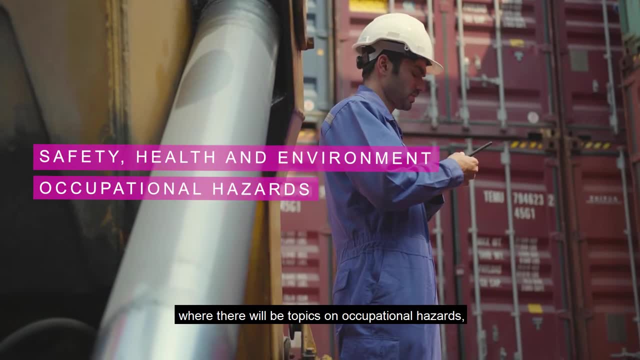 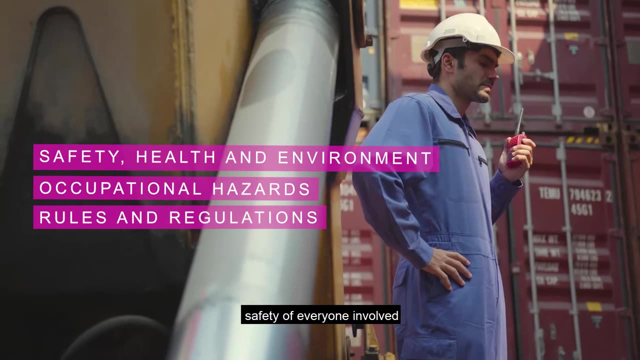 on public health and safety. In the module of environmental engineering, there are courses such as safety, health and environment, where there will be topics on occupational hazards, rules and regulations set by the government to protect the wellbeing and safety of everyone involved in a project. 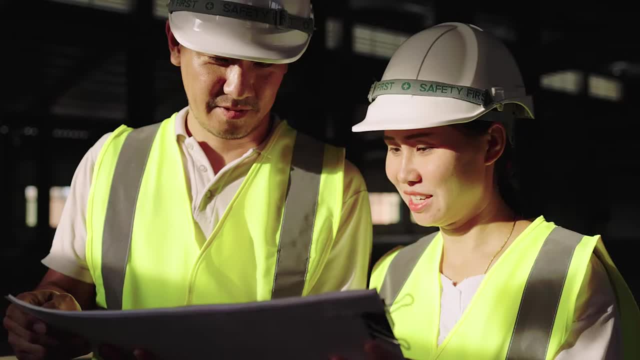 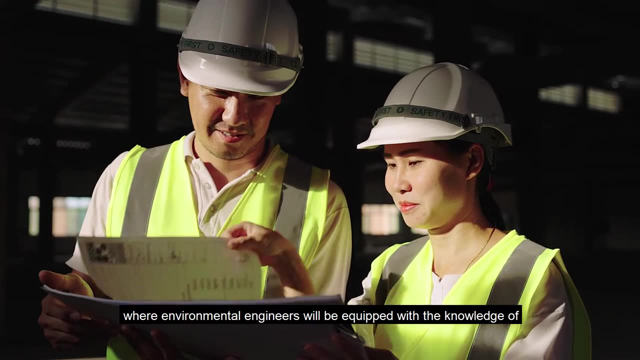 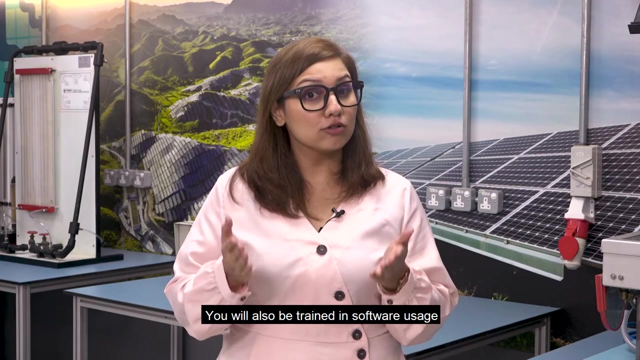 or workplace. Besides that, there is also a course known as safety process and risk management, where environmental engineers will be equipped with knowledge of marine and coastal major safety categories and ability to handle risks in the industry. You will also be trained in software usage via the Environmental Software and Application Module.